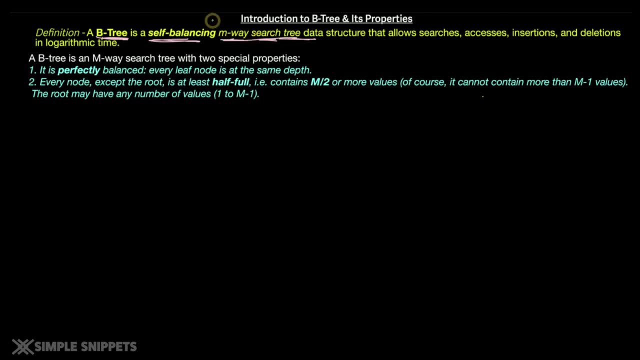 M-way search tree, but it is self-balancing in nature. This keyword is very important because this is what gives it a B-tree property. Now, if you don't know what is balancing, we have discussed what is balancing and why we need balancing and how we need balancing. 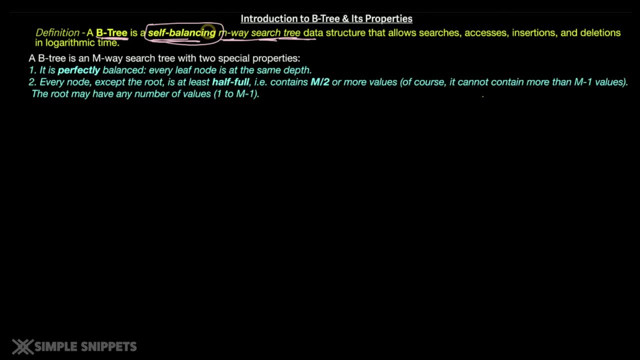 tree data structures make them more optimized and more efficient. I have those videos in this DSA playlist. Those are very, very critical. Do watch that, because when we were covering AVL tree, we required balancing right. So B-tree is a self-balancing M-way search tree. 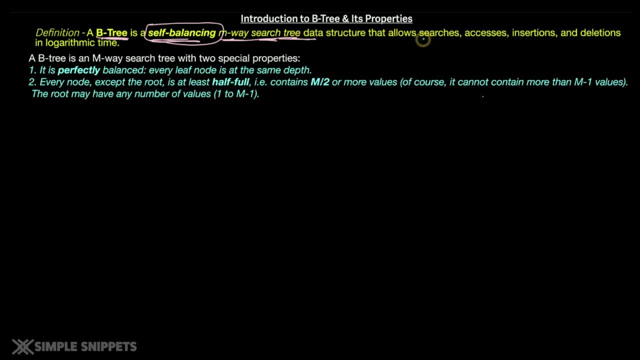 that allows searches, accesses, insertion and deletion operations in a logarithmic time. So this is the most efficient time when you want to do operations on tree data structure. B-tree: it has to be self-balanced or it has to be completely balanced, So a B-tree. 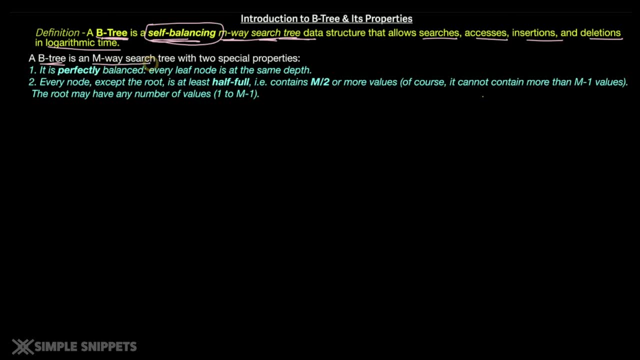 is again a M-way search tree with two extra special properties. So number one is: it is perfectly balanced. Keep this in mind. If you're making notes, you can take a note of this one. So basically, every leaf node is at the same depth. The next point is every. 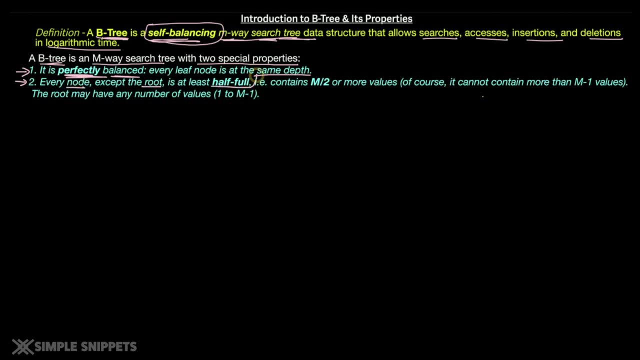 node, except the root node is at least half full, that is, it contains M by two or more values. So we know, since B-tree is a self-balancing tree, it has to be self-balanced or it has to be completely balanced. So a B-tree is again a M-way search tree with two extra special. 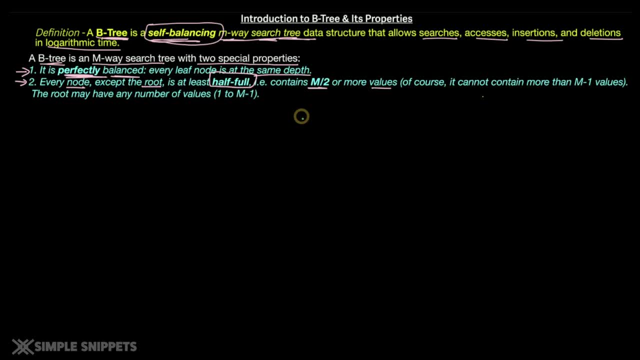 properties. So a B-tree is a self-balancing tree with two extra special properties. So let's say, if B is a M-way search tree and let's say if M equals to three, that would mean that one node can hold M minus one keys. right, The number of keys that one node can. 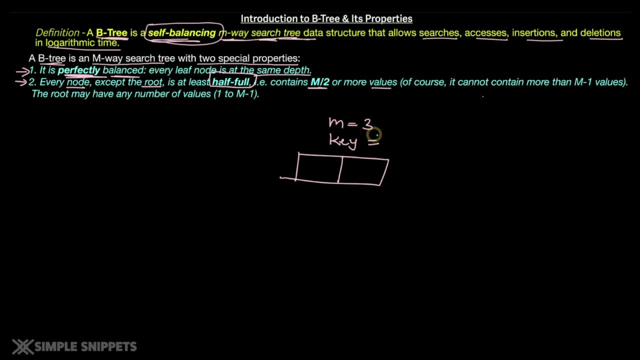 hold with M value three is M minus one, which is equal to two. So let's say this is node N1, it can hold two values, let's say 11 and 22.. So what this point is saying is every. 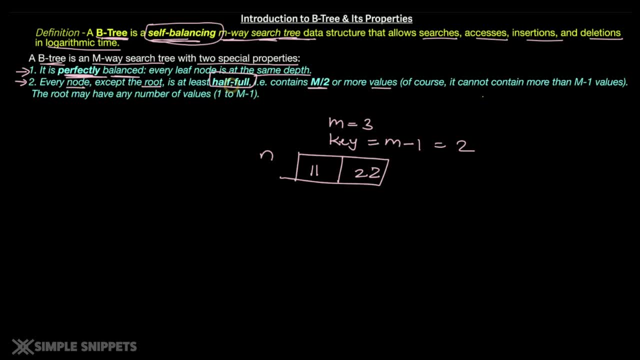 node, except the root node is at least half full, which means that this is valid. And if you have a number over here, then this is valid. but let's say the M is 4, it would mean that we can have M minus 1, that is, 3 keys. and if 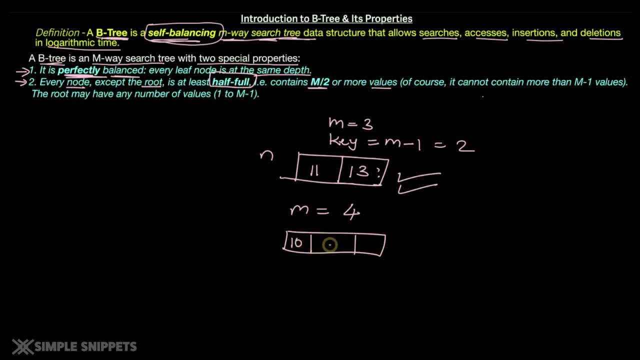 a node has, let's say, one value and two spaces are empty in that node. let's say, this is N2 and two spaces are empty, then this is not valid and it is not a B-tree. okay, So this is the only differentiating factor between a B-tree and a M-way search tree, because 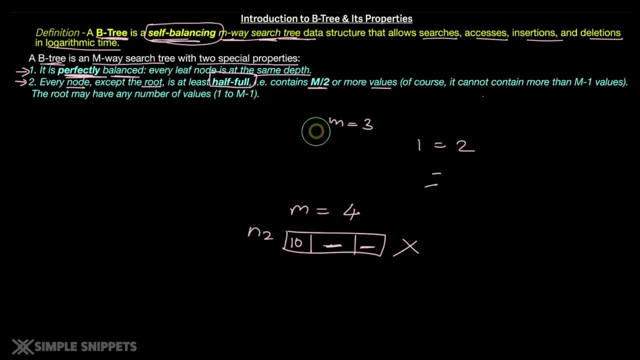 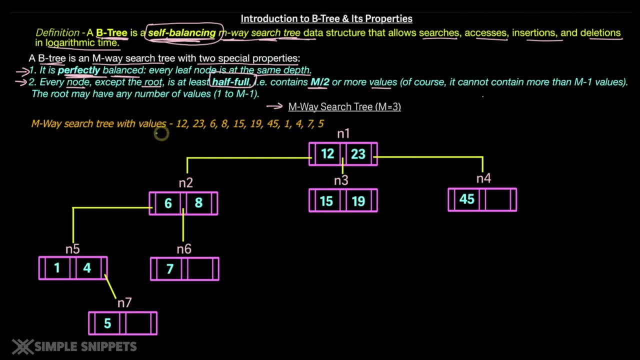 ultimately, B-tree is a M-way tree. B-tree is a M-way search tree with extra specialty which is related to the balancing. Now, to clear this out more visually, let's first take an example of a M-way search tree. okay, so this is a M-way search tree which is created using these values and we inserted 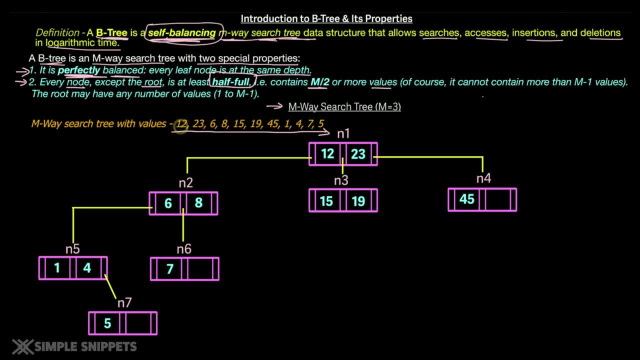 all these values one by one, from left to right. we've already discussed insertion and deletion in M-way search tree in previous video, hence I said you should watch that to understand the process. So when you create a M-way search tree with M equals to 3, which means that it can hold. 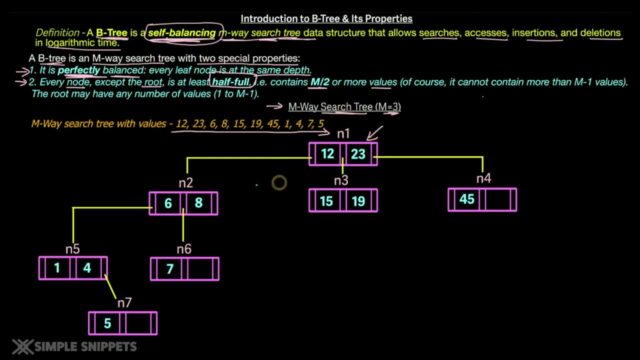 two keys and it can have three child. So you can see N1 has three children- N2,, N3 and N4- and it has two keys, 12 and 23.. So as the values came in 12, 23, we inserted them. when 6 came in, we went to the left of. 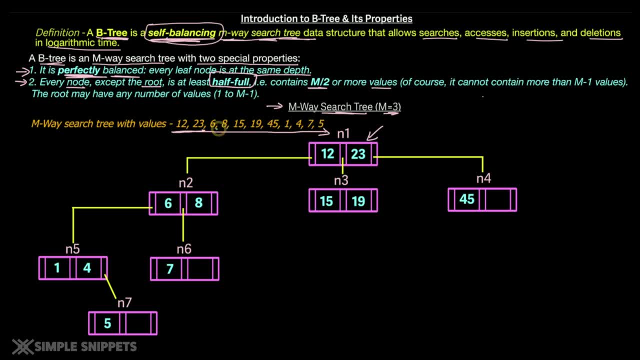 N1. then came 8,. 8 got accumulated over here. then came 15,. 15 is greater than 12, but smaller than 23. hence we created one new node in between them, and this process got us a M-way search tree which looks something like this: 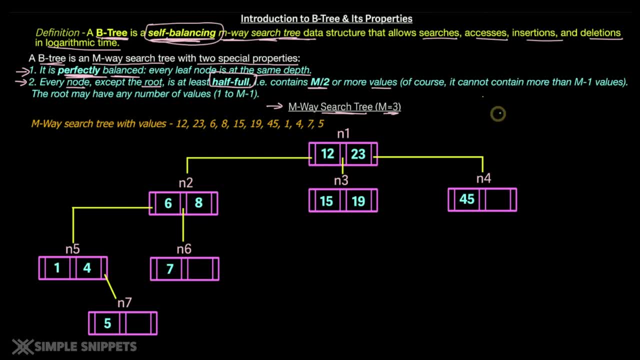 Now, if you observe this tree, is it balanced? It's not balanced. right In N1 you can see that we have the height of the left sub-tree as H equals to 1. I'm talking about this sub-tree and it has to be. H equals to 2. sorry, it's not 1, it's 2, because for this, 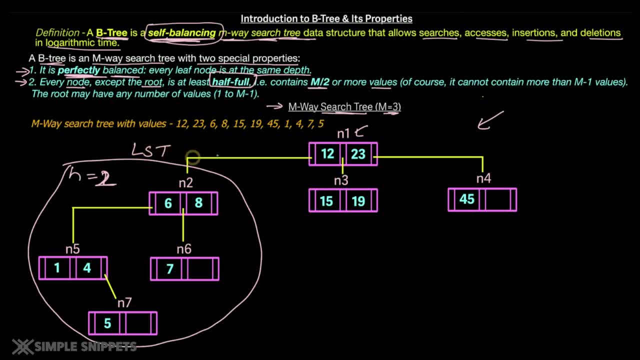 left sub-tree, that is for N1. what is the left sub-tree? this whole part, and the height is 2 because height is the longest distance between the root node of this left sub-tree, which is N2, and the leaf node N7 right. We have two links over here. 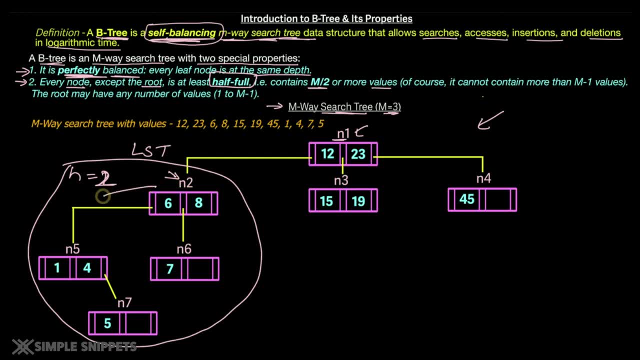 We go from N2 to N5 and we go from N5 to N7, so two hops are supposed to be made, that is, two levels. we have to go down and we have to go on the longest part to calculate the height. so height is 2, but for N1, what is the RST? the right sub-tree is this part and the 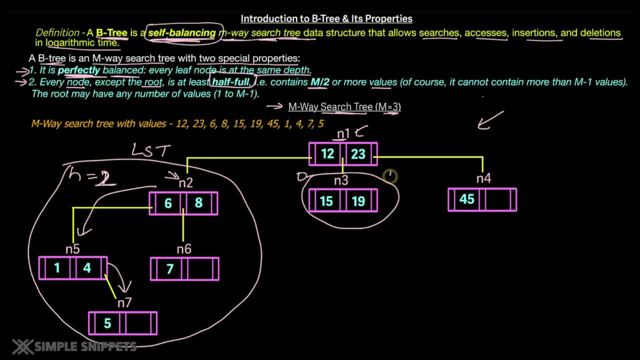 height over here is 0 correct because this is the RST and it is only a single standalone node on the right hand side of N1, which means that the height is 0. so you can see, if you subtract Height of LST minus height of RST, we will get 2 minus 0, which is equal to 2. so this 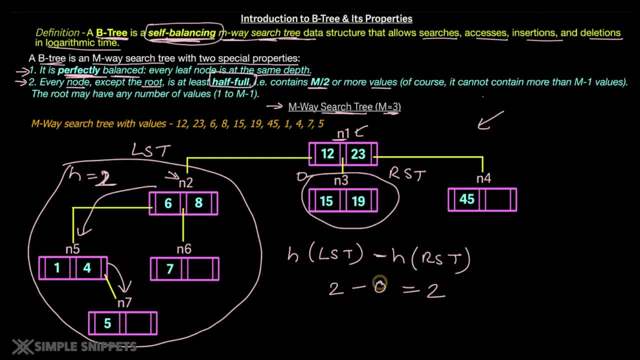 is not balanced because the height is greater than 0. if it's perfectly balanced, the height of left sub-tree minus height of right sub-tree is always going to be 0. okay, and this is only for perfectly balanced. so even though this is a m-way search tree, it is still not very. 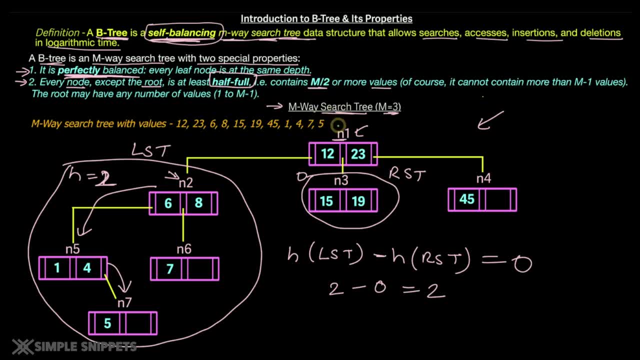 efficient because, as in when more and more values get added up, it will become more and more skewed. So the height of the tree is going to be in one direction, depending upon what the values are, and then the height between the left sub-tree and right sub-tree will keep on growing. and 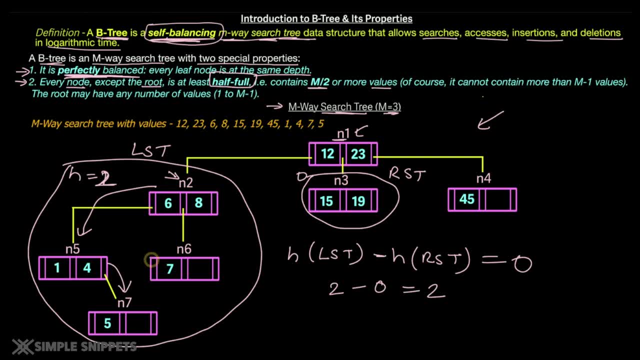 that will introduce inefficiency when you want to access a particular value. we've also discussed how an unbalanced tree is more inefficient compared to a balanced tree, right? so now let's take these same numbers, same values, and let's see how these same numbers will be represented. 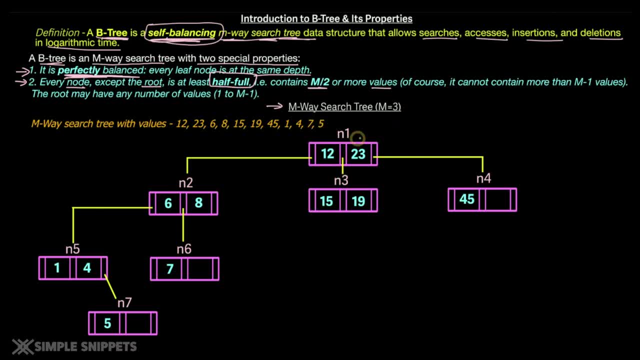 in a B tree, okay, so I would request you guys to just take a screenshot or just keep this diagram in mind. Now I'm going to switch to a B tree, which is made by these same values, in same order, but the structure is going to be different. okay, now, this is a B tree with, again, M equals. 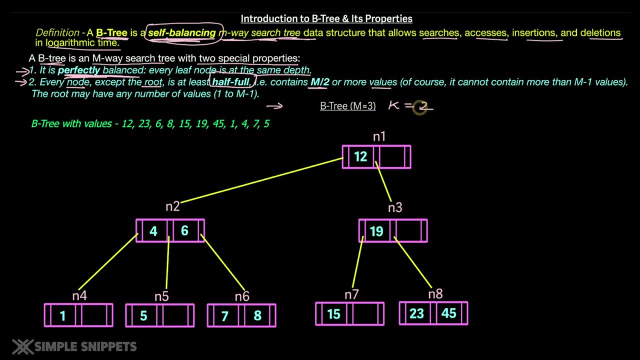 to 3, which means that the number of keys that one particular node will be storing is 2, which is M minus 1, and these are the same values. but you can see, now the structure is looking quite different and quite organized in a way, and now you can clearly see that it is properly. 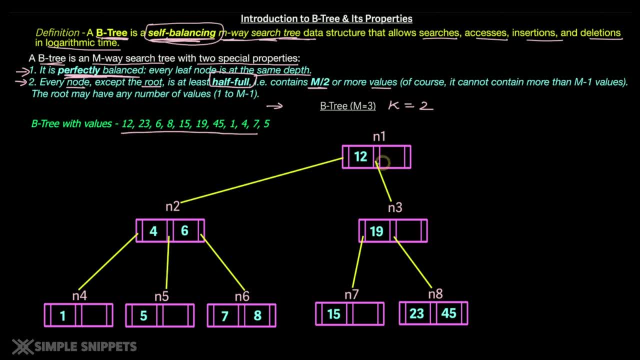 balanced as well. The numbers are same, But the insertion process In a B tree is different compared to a M way tree or M way search tree. we will discuss the insertion and deletion process in upcoming video, but right now we are just trying to understand how B tree is different compared to a M way search tree. 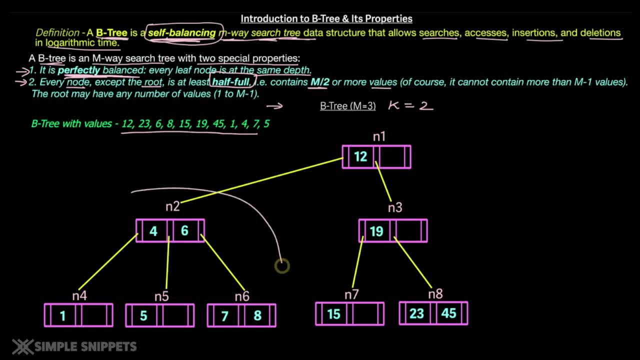 So if you now calculate the height of left sub-tree, which is this one, so for N1, the left sub-tree, is this and for N1, the right sub-tree, is this RST correct? the height of LST is going to be 1.. The height of RST is also going to be 1.. 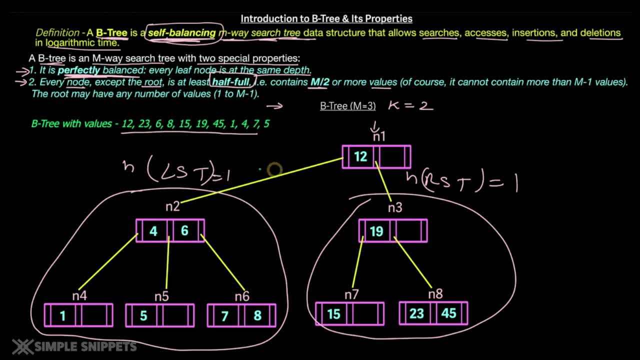 You can easily calculate and make out what is the height over here, and if you take a subtraction between the two, of course it is going to be 0 correct. So this means that it is perfectly balanced. What about the other rules that we just discussed? so we saw that a B tree is a M way search. 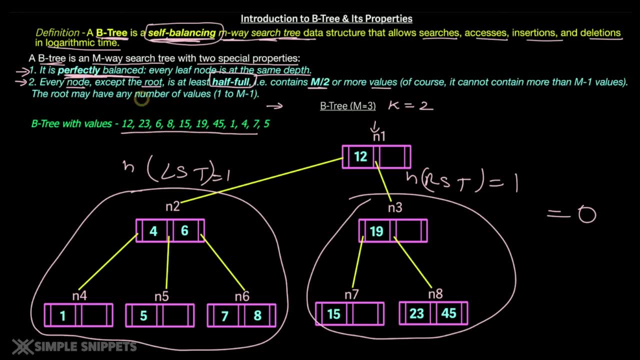 tree with two special properties, one is perfectly balanced. So what about this rule? that is, every node except the root node is at least half full. So let's take a look at the different nodes. so node N1 is the root node. how many number of keys? 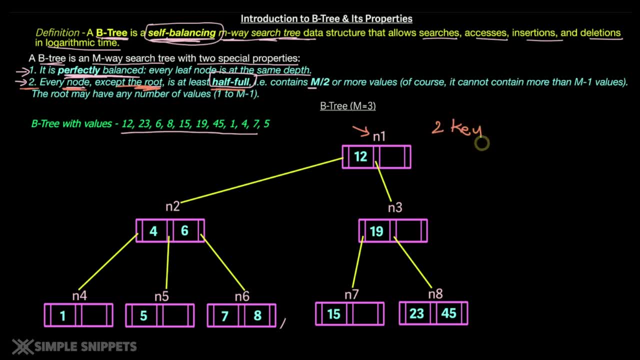 How many keys can it store? each node can store maximum two keys. How many are there? currently in N1 we have one key, so it is half full, correct? similarly, N2 is completely full, N3 is half full, N6 is full, N8 is full, N7, N5 and N4 are half full. 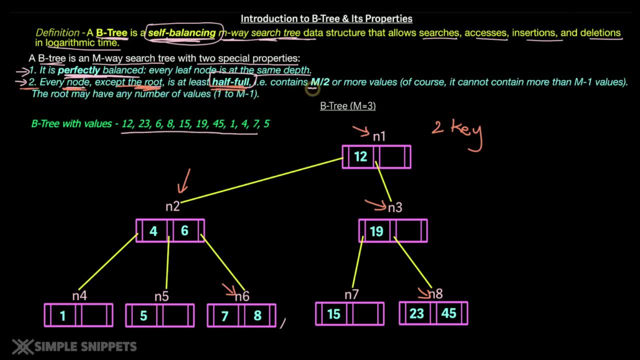 which means that every node, except the root node, is at least half full, which means each node contains M by 2 values. so M is nothing but 2. M by 2 is equal to 2 by 2, which is equal to 1. So every node at least has one particular key inside it. so this condition is also true. 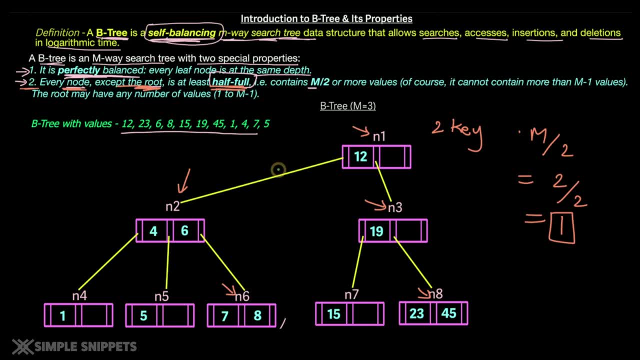 hence now you can say that this is a proper B tree. So this was the main difference between B tree and M way search tree. again to reiterate, B tree is also a M way tree with two special properties. one of them is self balancing and the other one is that every node, except the root node, has to be at least half full. 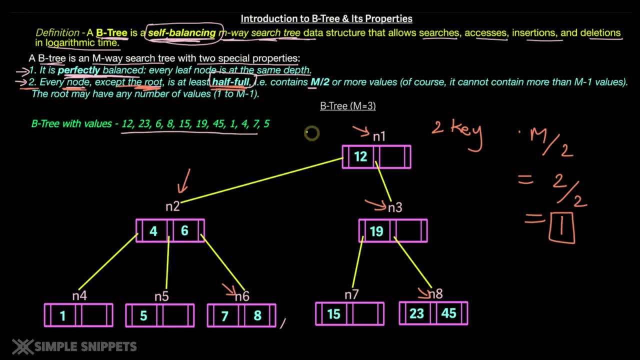 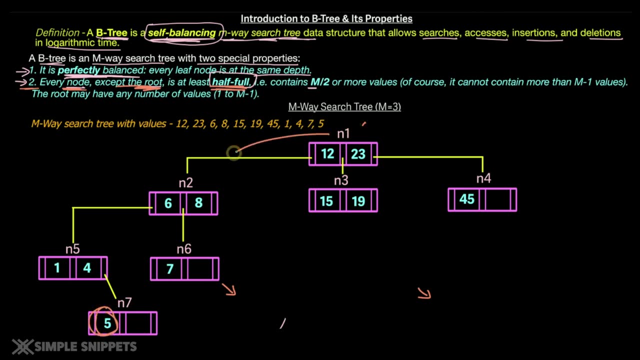 So this is much more efficient compared to the M way search tree because it is balanced And just to give you an example, with the existing two trees that we just saw. again, switching back to M way tree, If you were to find the value 5, starting from root node N1, you will go to N2. you will then. 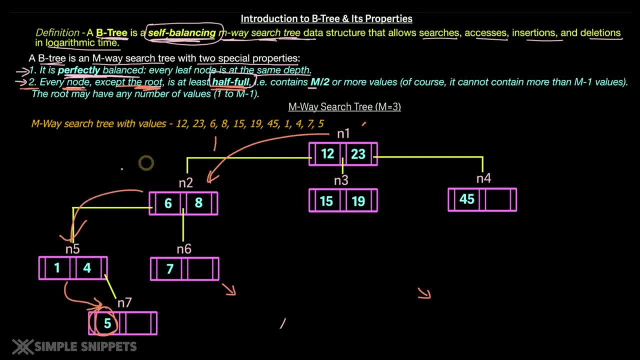 go to N5 and then you will go to N7, right, so you need 1, 2 and 3 hops, but same if you compare for B tree. let's say again you want to search 5 in a B tree. in that case you only. 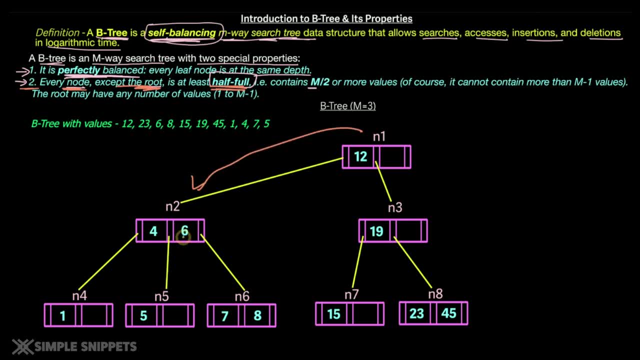 need 2 hops. You will start from N1, you will go to N2, from N2 you will go to N5 and you've got your answer. So you can see more the imbalance of a tree, more time it is required to search or you. 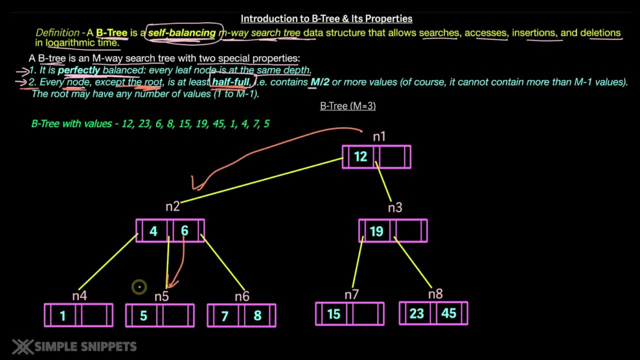 know, access a particular data value inside the tree. if the tree is perfectly balanced, the number of hops required or number of levels that you require to go find that number or find that key value is less, which means that it is faster. okay, so, lastly, just talking about 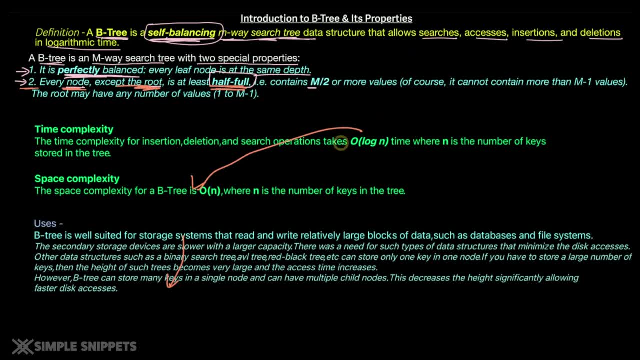 the uses, And you know it's space and time complexity. we've already discussed what is space complexity, what is time complexity in two dedicated videos. those are also very important. please watch them. the time complexity for insertion, deletion and search operations takes O time, and this is probably the more, and this is highly efficient for those who know what is time complexity. 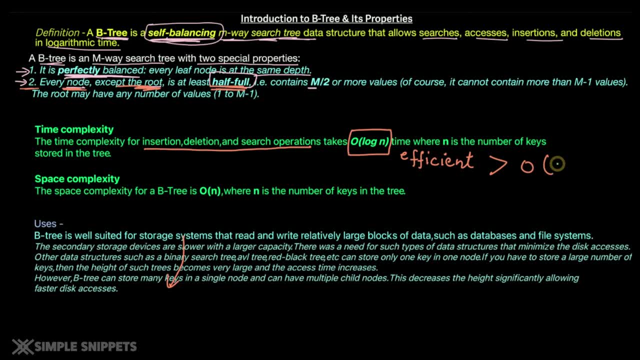 this is much more efficient compared to O, that is linear time. okay, so N is the number of keys stored in the tree. Okay, Not the number of nodes, but the number of keys. okay, the space complexity of a B-tree is O of N, which is where N is the number of keys- again, not node, but the actual number. 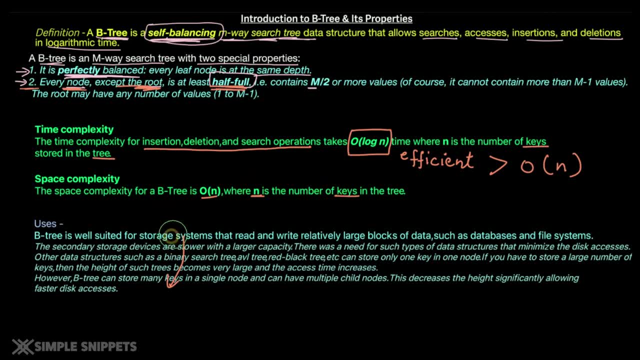 of keys inside every node. and lastly, to talk about its uses, B-tree is actually well suited for storage systems that read and write relatively large block of data. such examples are databases and file systems- and the reason why it is more suited is because the secondary storage 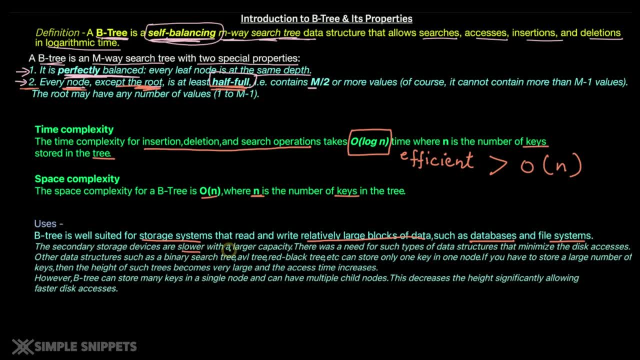 for example, your hard disk drive, or SSD, Is much more slower, with large capacity, compared to a main memory like RAM. right, so there was a need for such type of data structures. that minimizes the disk access. so structures like binary search tree, AVL tree etc. can store only one key in a particular node. but if you 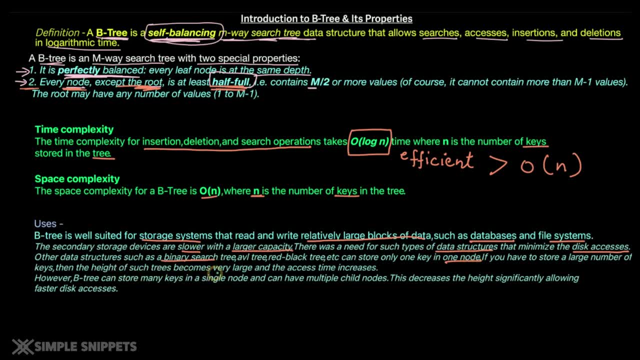 have to store a large number of keys, then the height of such tree becomes very large. right. in a binary tree you can have one key per node, but in a B-tree you can have many number of keys in one single node. Okay, And since B-tree is also a balanced tree, the access time is also very less. I just demonstrated. 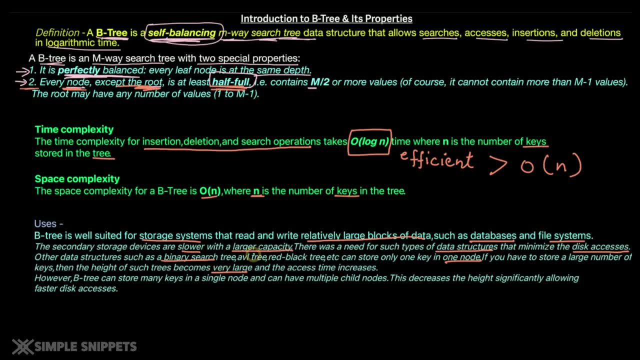 that in the previous example where we compared, the access time was more in M-way search tree compared to the B-tree right. so since B-tree can store many keys in a single node and can have multiple child nodes, this decreases the height significantly, allowing faster disk access. this is exactly what we just demonstrated in our two examples. 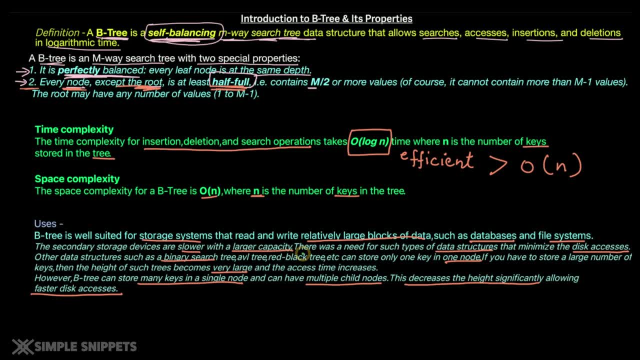 So this was a quick introduction, guys, to B-tree. You guys can note down these nodes if you are taking them down for your exams or something like that, just for theoretical purposes. In the next video we will see the insertion process of B-tree and also the deletion process. 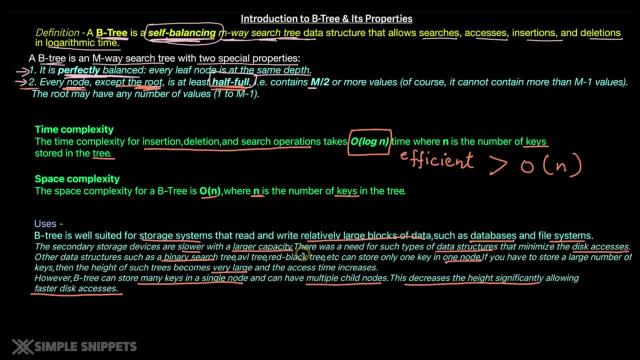 compared to M-way search tree. okay, because both of them are different, because the self balancing factor operation has to be done in B-tree. Okay, so I'm going to wrap up this quick intro video over here. I hope you understood what is B-tree. let me know in the comments if you understood this video. if you have any queries. 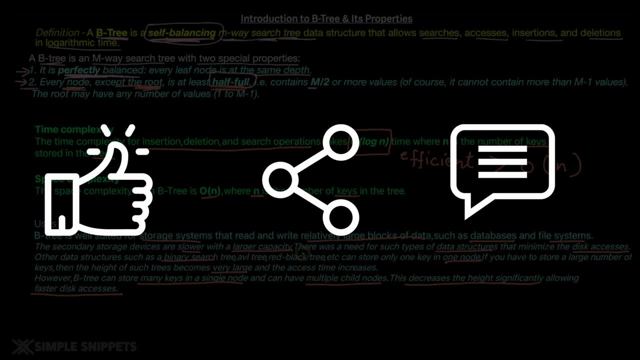 give a thumbs up to this video. if you like this video, please share it with your friends. I will see you in the next video. bye, bye, Aditya, friends, and I'll see you guys in the next one. peace. 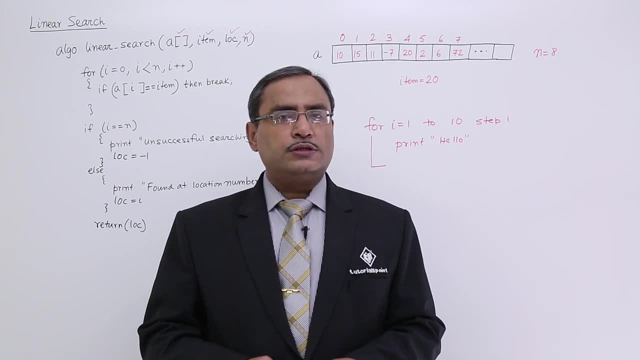 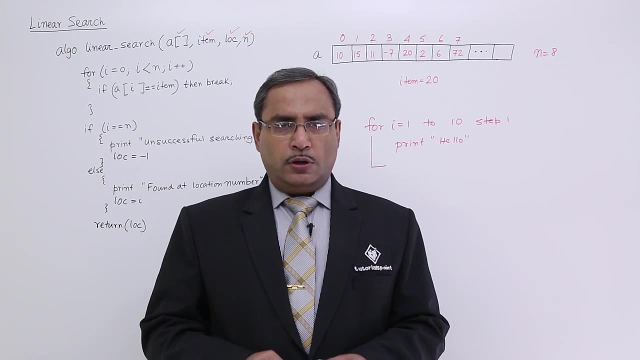 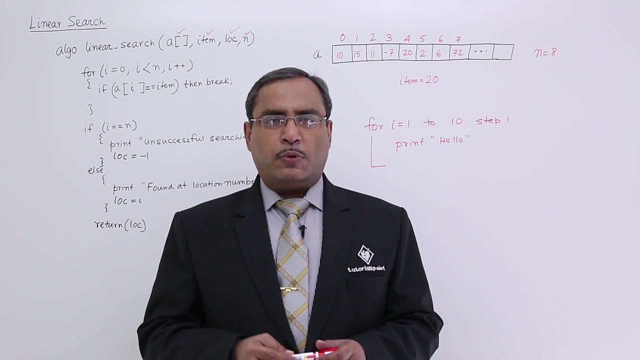 In this session we are discussing linear search or sequential search. In this particular searching algorithm, we will be searching for a search item on an array which is containing, say, n number of data. Let us suppose the array is containing n number of data starting from the subscript. 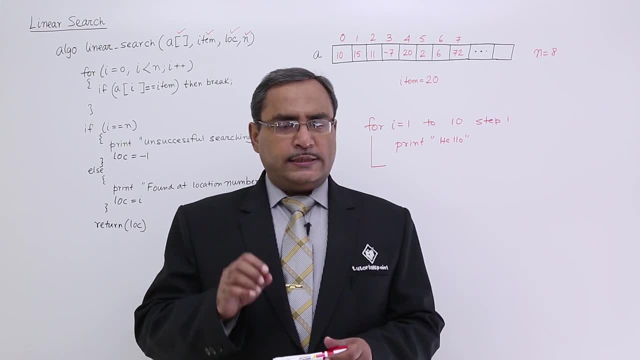 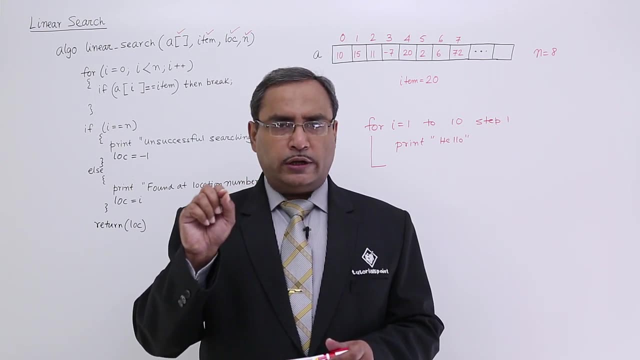 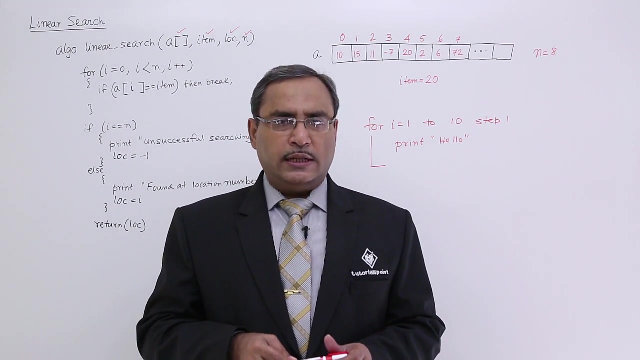 number, 0 to n minus 1.. I shall search for a certain item, say 100, and that item will be searched in each and every locations content starting from 0 to n minus 1.. If I can get the data in any one of the locations, then I shall find that successful searching has taken place. 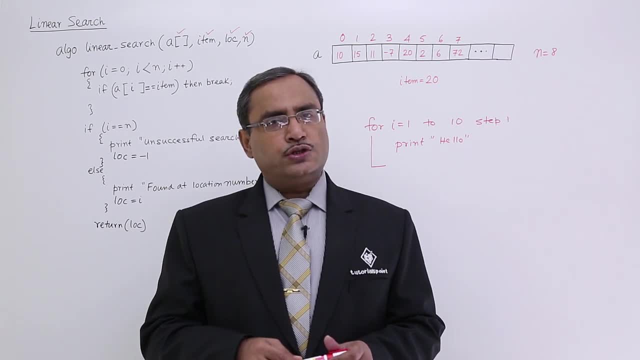 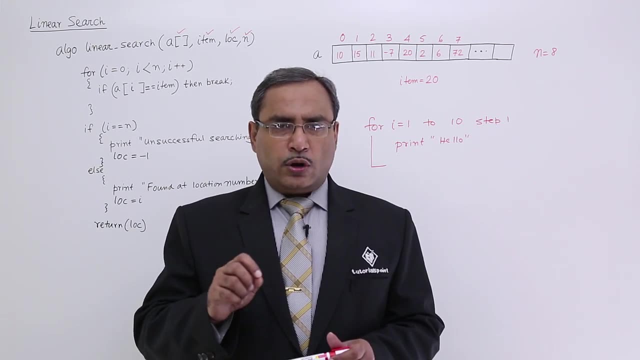 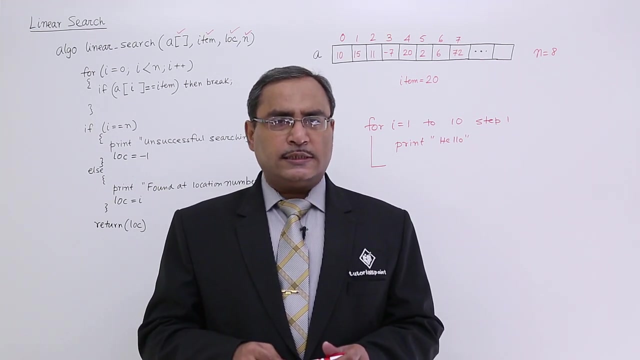 and I shall print the location number. and also I shall return the location number where the successful searching has been done. But if in the locations 0 to n minus 1, if I can't find the item in the case, I shall print unsuccessful searching and I shall return the value minus 1.. Why minus 1? Because minus 1 is. 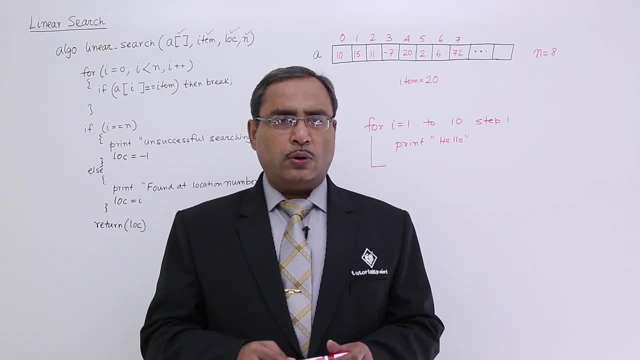 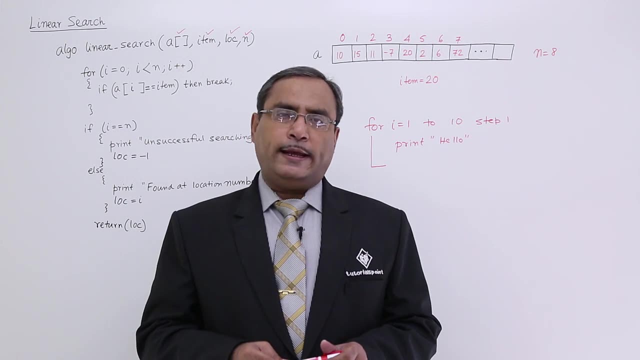 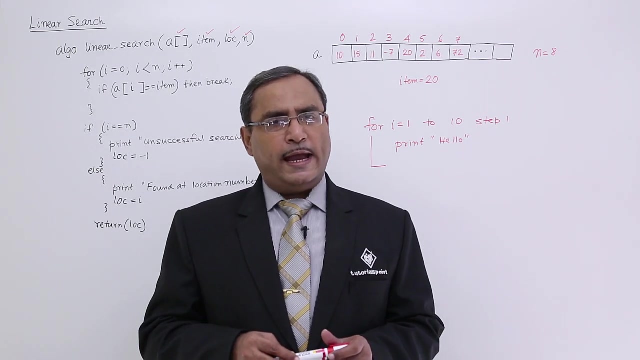 not a valid subscript or location number, because the location numbers are ranging in between 0 to n minus 1.. In this way, this linear search operation will take place. So now, in this particular case, we know that the maximum number of searching which will be required will be n? n number of.